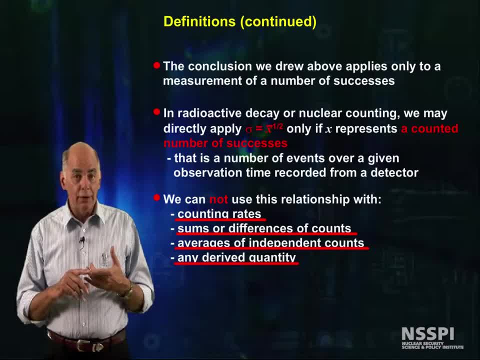 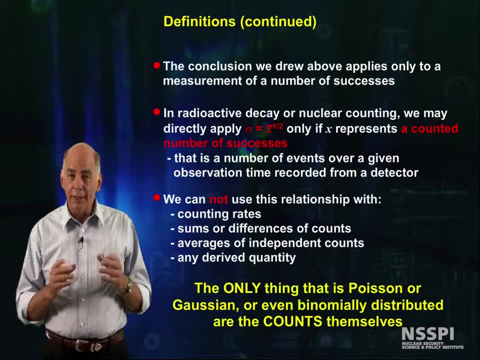 or if it is a number of events over a given observation time, and therefore, even if the number of successes is the same, we shouldn't then be using this formula for all the kinds of values, and not all of them are the same. 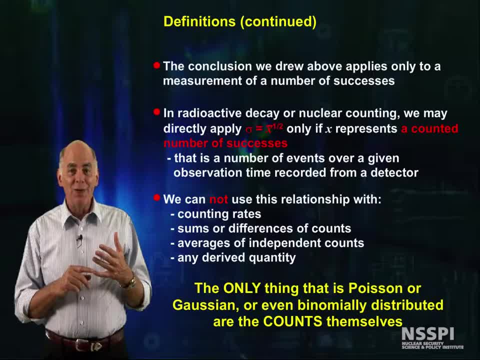 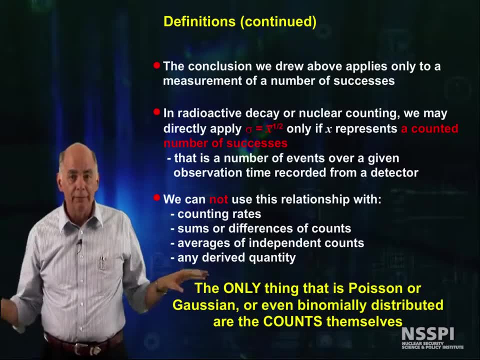 The solution to this question, though, is that the number of successes is zero. The number of successes is zero, That's all. The answer to this is: counts themselves, That's it. As soon as you add them, subtract them, multiply them together. 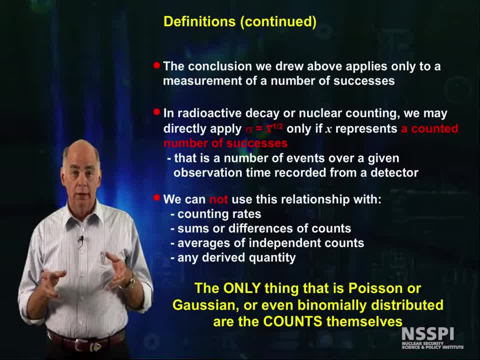 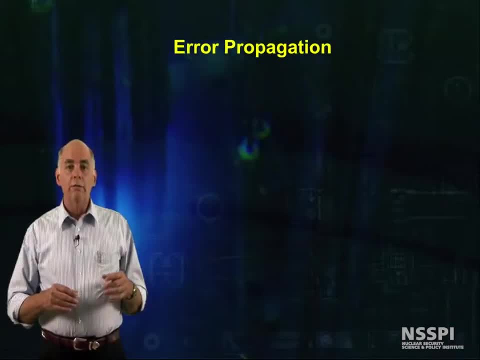 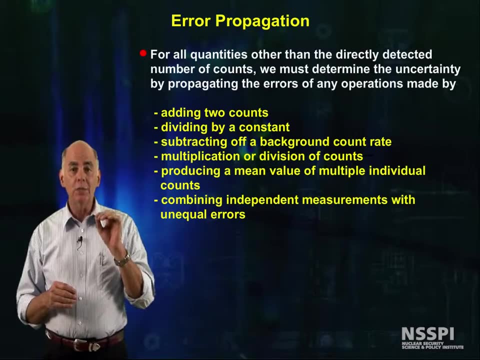 multiply by a constant, divide them or even look at them hard. all bets are off. Well, what are we going to do? Fear, not Help is on the way For all quantities other than the directly detected number of counts. we can determine the uncertainty by propagating the. 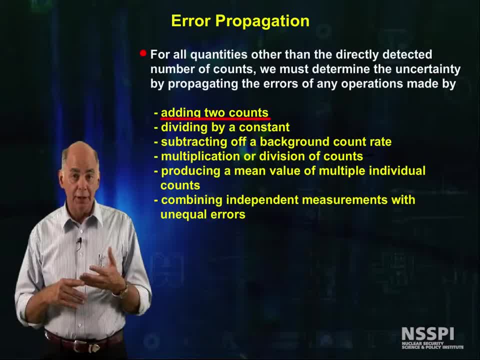 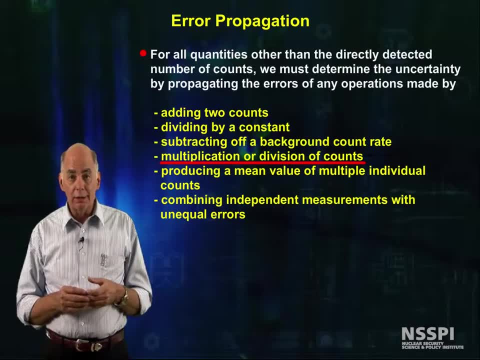 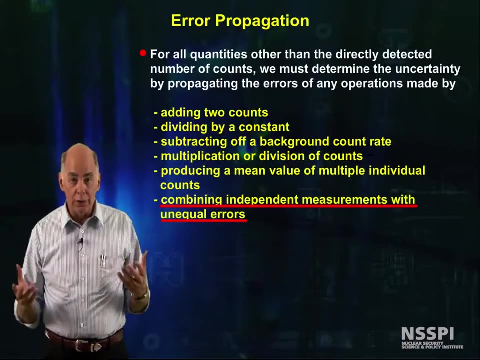 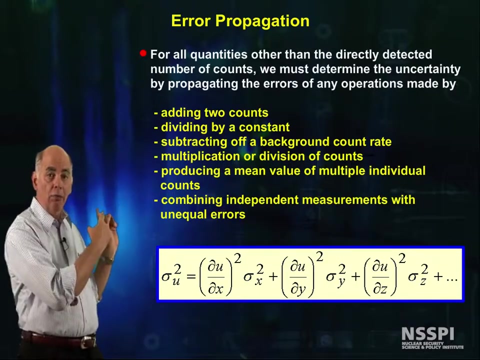 errors of any of these operations made by adding two counts, dividing by a constant, subtracting off a background count rate, multiplication or division of counts, producing a mean value of multiple independent counts, combining independent measures with unequal errors. To do these mathematical feats we need to use the error propagation formula. 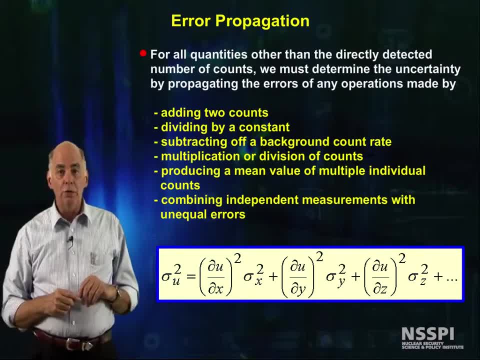 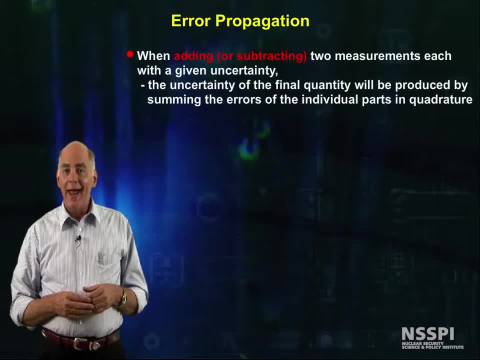 shown here. For those of you who actually know what the backward 6 means, you can easily derive what I'm going to show you next. When you're adding or subtracting two measurements, each with a given uncertainty. the uncertainty of the final quantity will be produced by summing of the errors of the individual parts. 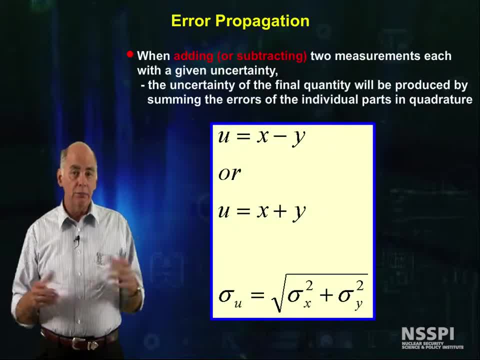 squared, Or if x and y is summed or subtracted to produce u, then the standard deviation in u is the square root of the sum of the standard deviations of x and y each squared. As a side note, now you can see why statisticians love variance. Said their way, the variance of 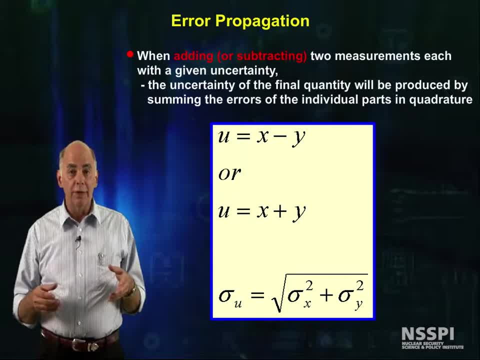 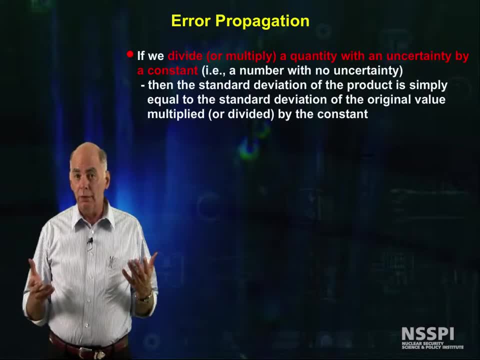 u, the sum is equal to the sum of the variance of x and the variance of y. Well, what if we multiply a count by a constant? If we divide our multiply a quantity with a known uncertainty by a constant, that is a number with no uncertainty.